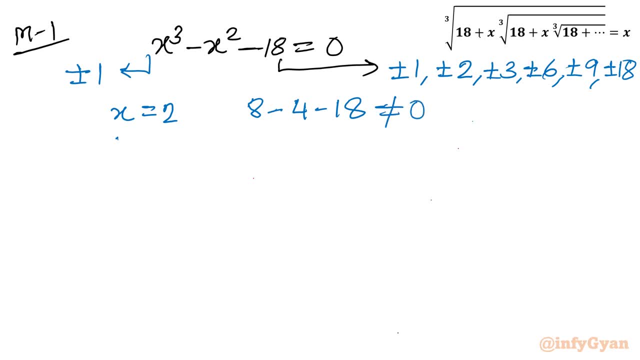 Is this equal to 0? No, it is not. Let us put one more positive value: x is equal to 3.. Then you will write 3 cube minus 3, square minus 18.. Is this 0?? Yes, 27 minus 9 minus 18.. 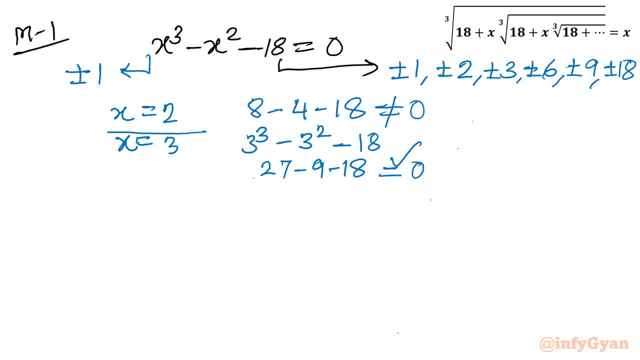 Yes, it is equal to 0. That means x is equal to 3 is our base solution. Now I will use synthetic division method to find out what is the ratio. of x is equal to 3 to x is equal to 3.. 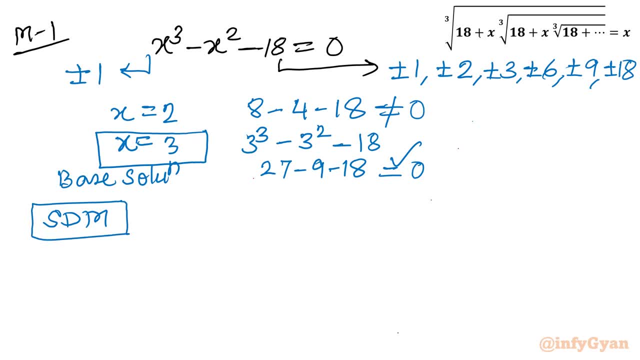 The remaining two roots also. So let me write all the coefficients of this cubic equation. So the coefficient of x, cube 1,. coefficient of x, square minus 1,. coefficient of x- it is not there, so 0.. Constant coefficient minus 18.. Now I will put one line over there. 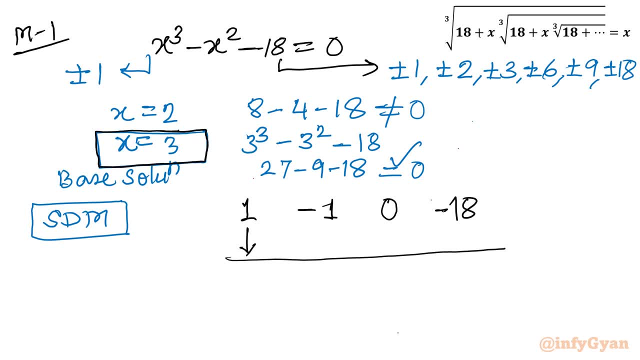 Our base solution is: x is equal to 3.. I will write leading coefficient as it is: 1.. Now, 3 times 1, 3, 2.. 3 times 2, 6, 6.. 6 times 3, 18.. 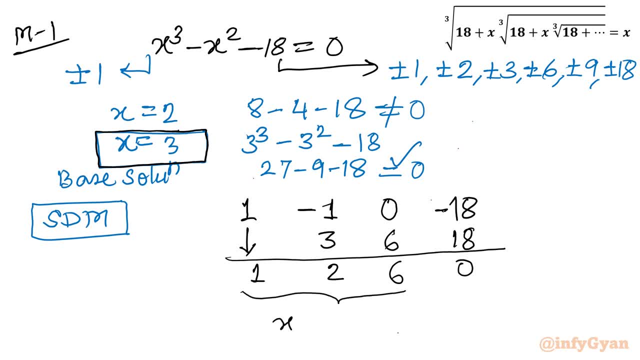 Now 1, 2 and 6 basically are the coefficients for quadratic equation: x square plus 2x plus 6.. Now we will solve this equation to get the remaining two solutions. One solution is clear, It is: x is equal to 3, which is our first base solution. 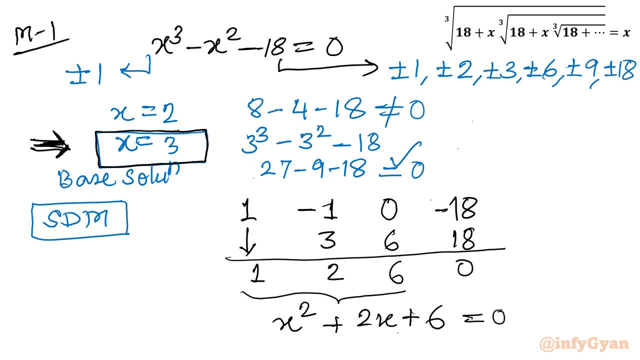 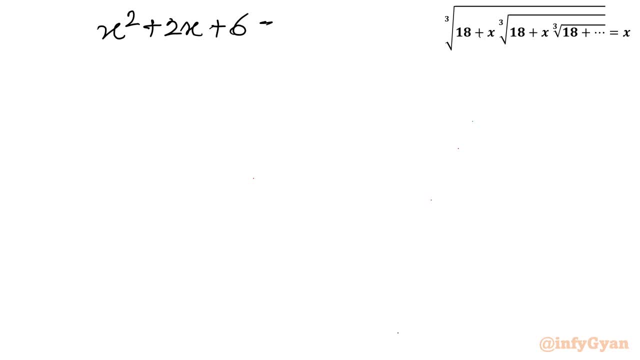 Let me solve this equation: x square plus 2x plus 6, equal to 0.. x square plus 2x plus 6, equal to 0.. Let us apply Sridharachara formula or quadratic formula: x is equal to minus b, so minus 2, plus minus under the root b square, so 2 square. 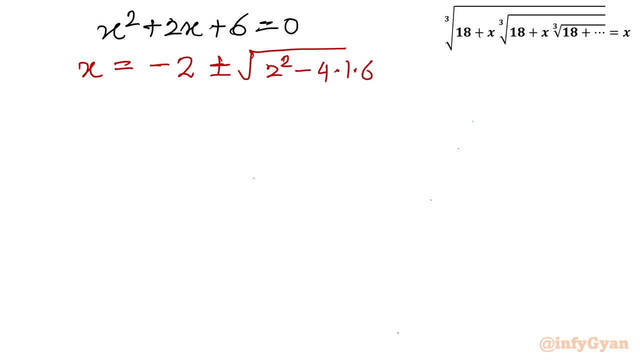 minus 4 times 1 times 6 divided by 2a, a is 1.. So 2. minus 2 plus minus under the root 2 square is 4. minus 24 divided by 2. Now you will write minus 2 plus minus square root of negative 20 divided by 2.. 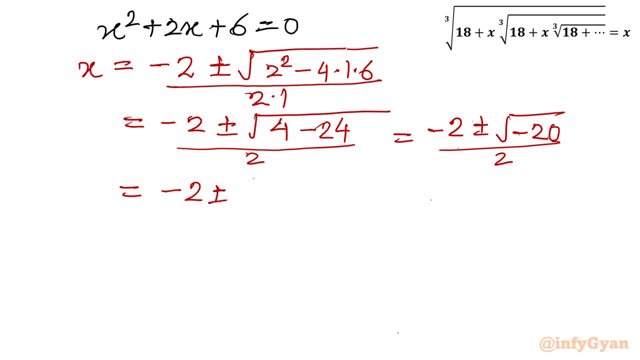 Here we can consider: minus 2 plus minus 20 is 4 root 4 times 5, so 2 root 5. we will write. So 2 root 5, we will write. So 2 root 5, we will write. 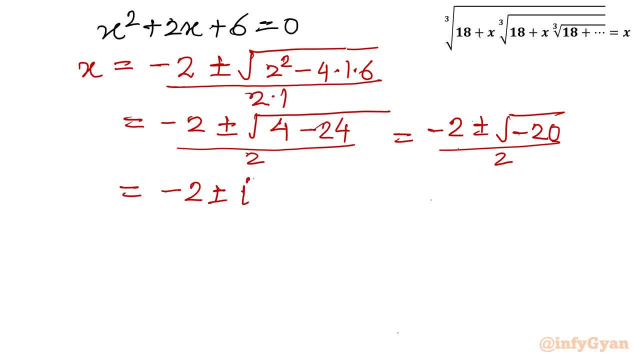 And square root minus 1 is i, So we can write it as i: times: 2 square root 5 divided by 2.. Divide with 2. Minus 1 plus minus i root 5.. Complex solution, So we will reject it. 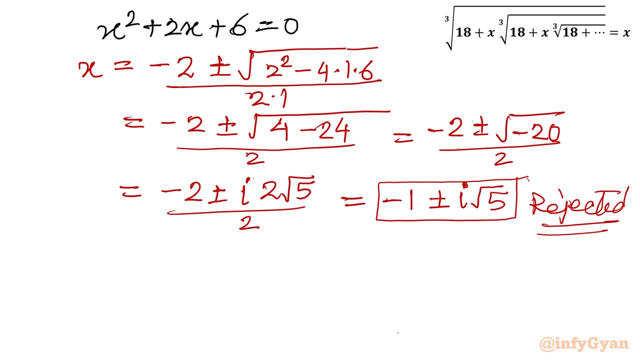 Rejected. Now let us consider method number 2.. Method number 2 is Using algebraic manipulation and using the algebraic identities method. So let me write our equation once: x cube minus x square equal to 18.. Now I will split 18 as x cube minus x square. as it is. 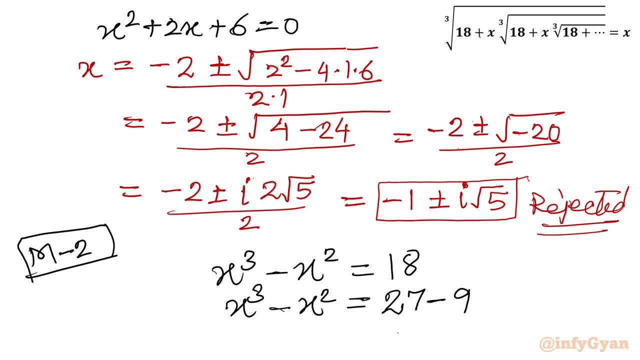 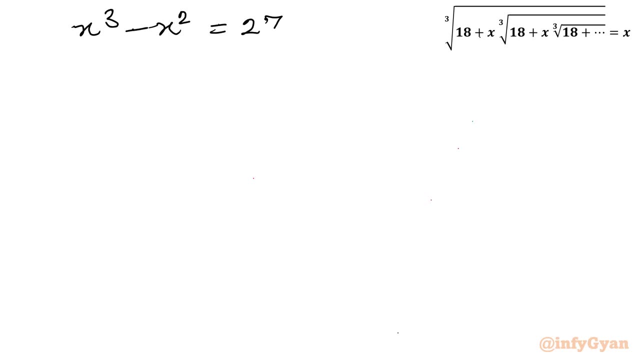 18, we can write 27 minus 9.. Now I will consider 27 to the left and 9 to the left. See how it would be. Let me write once: x cube minus x square is equal to 27 minus 9.. 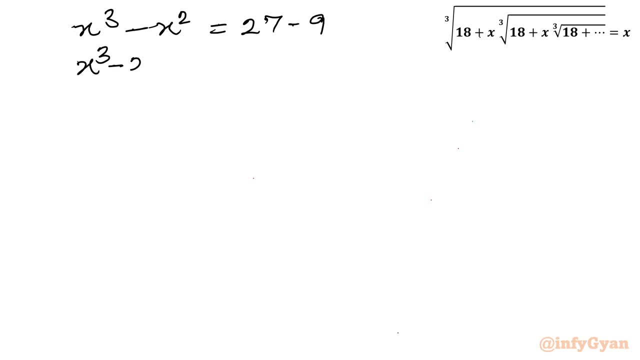 So I will write x cube minus 27.. Then I will consider minus x square plus 9 equal to 0.. Now you can see it is x cube minus 3 cube and minus sign. Let us consider minus common, So x square minus 3 cube. 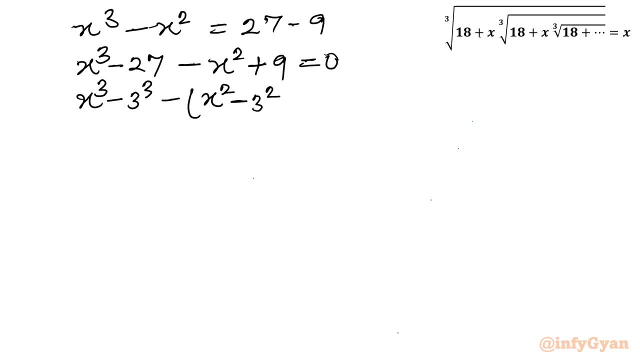 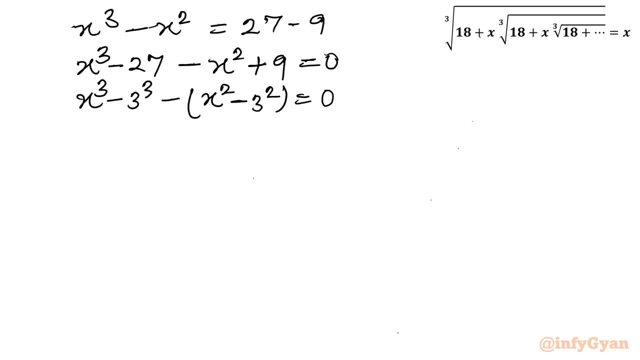 And second is difference of two squares: a square minus b square. Let us apply a minus b, a square plus b square plus ab, So 3x plus 9.. Now come to the difference of two squares: a square minus b square.